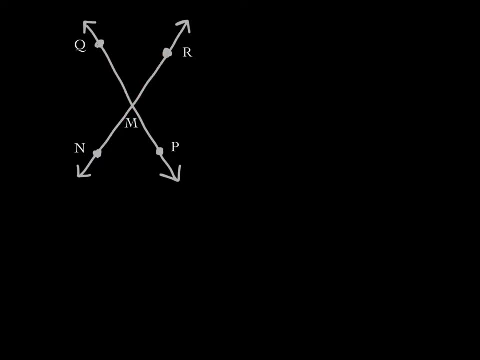 The pair of angles NMP and RMQ are called vertical angles And vertical angles have equal measures. And notice: we have another pair of vertical angles: NMQ and PMR are also vertical angles, so they have equal measures. So we have this angle here, right? 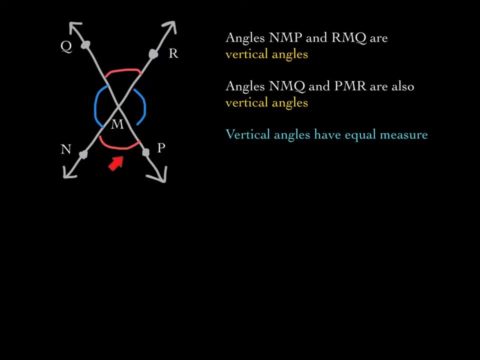 Is equivalent to this angle here, That is, RMQ is equal measure with NMP. Same thing here: NMQ is equivalent to PMR. Awesome, Now, if we have a pair of parallel lines right, Meaning they never intersect each other. 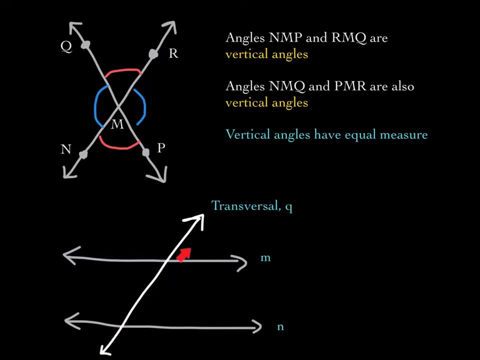 And we have this third line that cuts through Or intersects the pair of parallel lines. This line here is called the transversal. I'm naming the transversal Q And I'm naming the parallel lines M and N, When a transversal here intersects a pair of parallel lines. 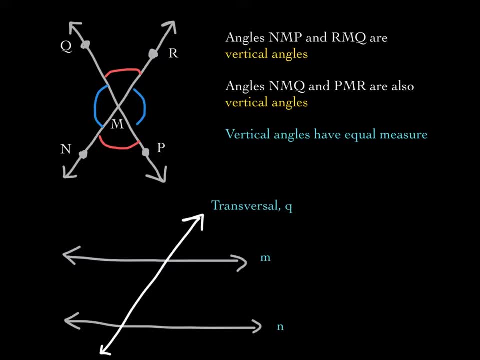 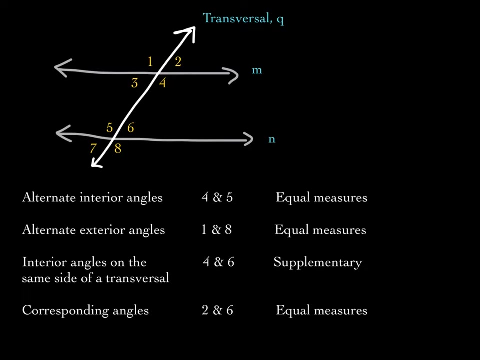 it forms eight angles. Now we know from geometry that angles 1 through 8 have some special properties, So I'm about to go through some special properties here that exist between these angles. So we have alternate interior angles. Four and five are examples of alternate interior angles. 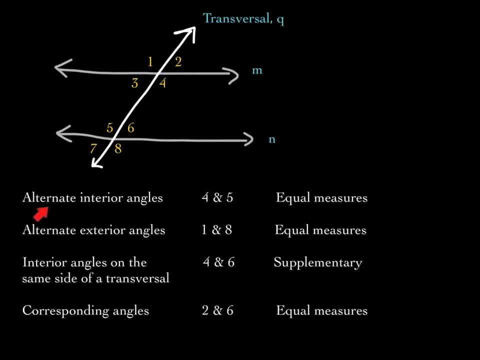 Now, when you hear the word alternate, think opposite sides of the transversal. So alternate right, Opposite sides of the transversal And interior, meaning that they are within the parallel lines. This is a parallel line M, parallel line N. 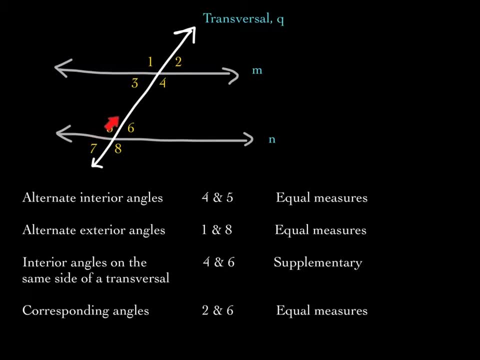 And they are both within the parallel lines. So alternate interior angles And they have the same measure. Angles 3 and 6 are also alternate interior angles. Alternate exterior angles are 1 and 8. Alternate they are on opposite sides of the transversal. 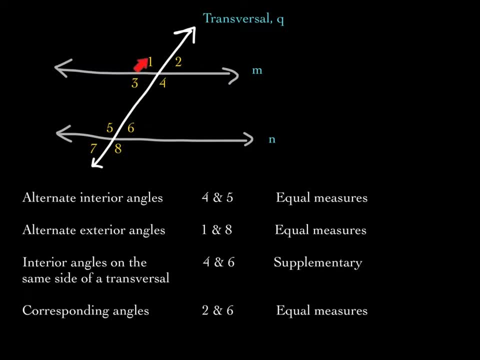 And exterior because they are without the on the outside of the parallel lines. So these are equal measure. Angles 2 and 7 are also alternate exterior angles, Interior angles on the same side of a transversal, So that would be 4 and 6.. 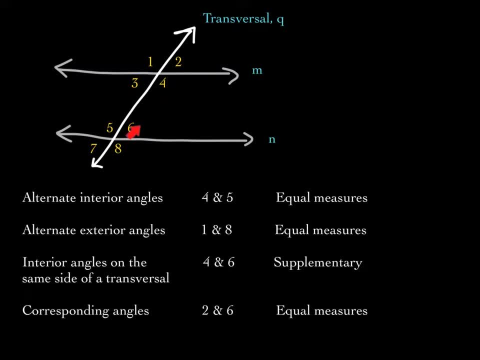 They are interior angles on the same side of the transversal. Now they are not equal, They are supplementary, So they sum to 180 degrees. The same is the case for angles 3 and 5.. Finally, corresponding angles like 2 and 6,. 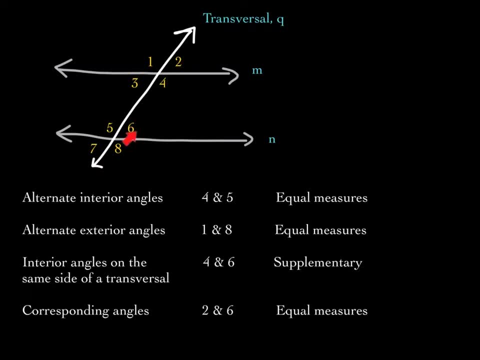 are on the same side of the transversal And they are both above the parallel lines. Look at this: 2 is above angle 2 is above line M And angle 6 is above line N. So these are corresponding angles. 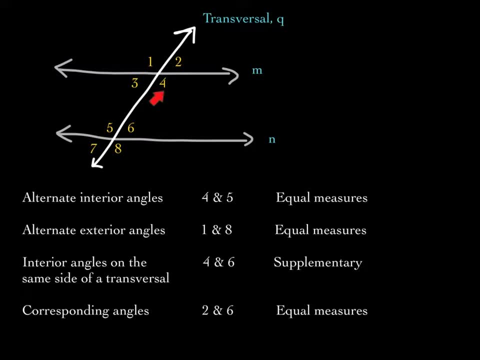 And they are equal. Angles 4 and 8 would also be corresponding angles. They are on the same side of the transversal And they are both bent. They are both beneath the parallel lines. There are a lot of corresponding angles. 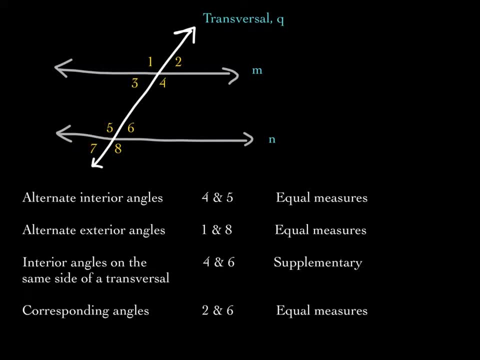 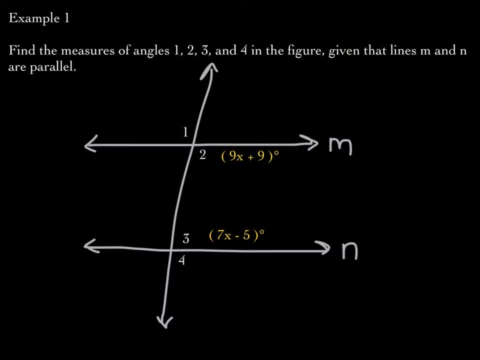 Like: 1 and 5 would be corresponding, 3 and 7 would be corresponding, And corresponding angles have equal measures. Alright, example 1. Find the measures of angles 1,, 2,, 3, and 4 in this figure. 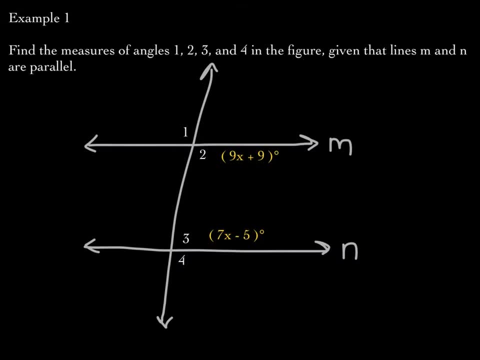 given that the lines M and N are parallel. Now, the first thing I notice is that angles 2 and 3 are interior angles And they are on the same side of the transversal, And we just mentioned that interior angles on the same side of the transversal are supplementary. 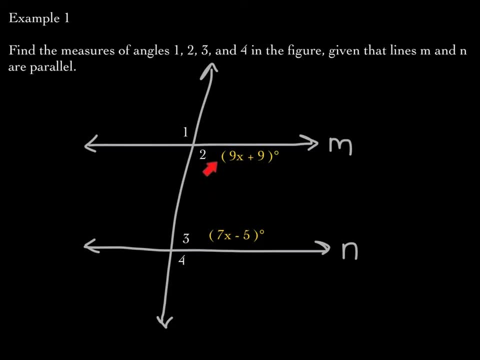 That means they sum to 180 degrees. So what I'm going to do is I'm going to set up like a little equation. I'm going to say 9x plus 9 plus 7x minus 5 is equal to 180. 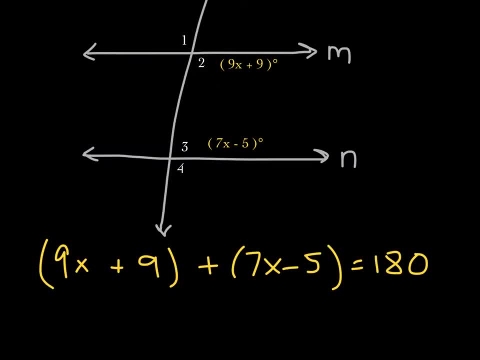 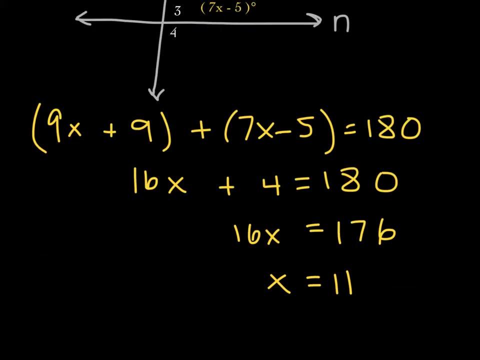 Remember that supplementary means angles that add to 180 degrees. So you can see, then this leads us to 16 plus 4 is equal to 180.. And then, of course, subtracting 4 from both sides leads us to 16x is equal to 176. 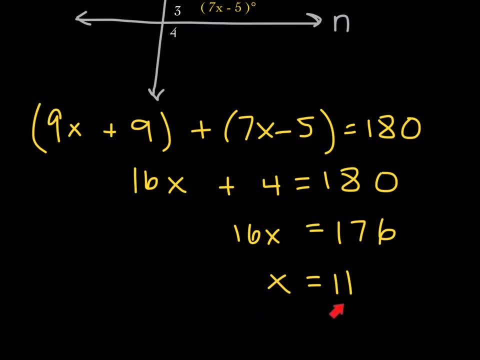 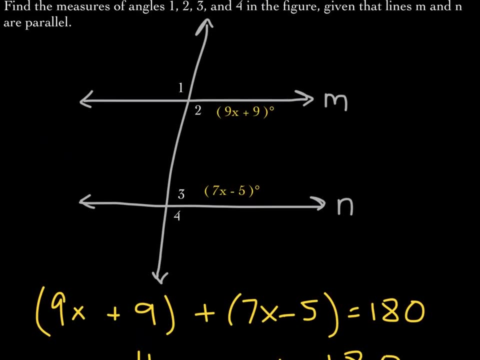 Dividing both sides by 16 gives us 11.. Now x is equal to 11.. What I'm going to do is go back to my figure And I am going to basically plug 11 in, And that will give me the measure of angle 3.. 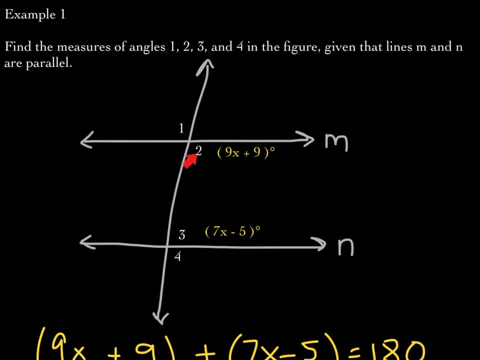 And the measure of angle 2.. And then notice that 1 and 2 are vertical angles, So they're going to be equal. So whatever I figure out for angle 2 will be the same measure for angle 1.. 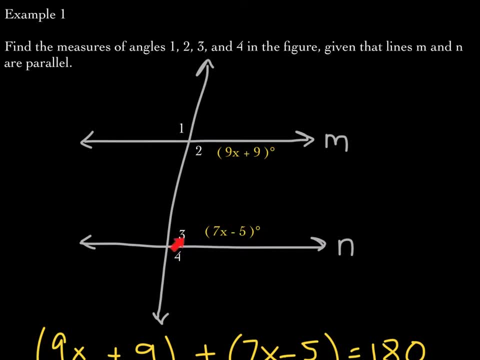 And let's see: Angle 1 and angle 4 are alternate exterior angles, So 1 and 4 are also equal. So basically, once I find the measure of angle 2, that's going to give me the measure of angles 1 and 4 as well. 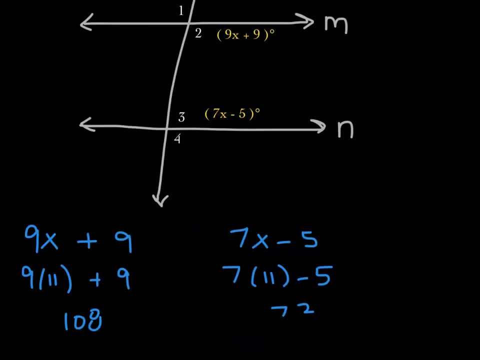 Okay, folks, I plugged 11 in, both into this expression and into this expression. So I found that angle 2 is measured at 108 degrees. So that will be the measure of angle 2.. Also the measure of angle 1.. 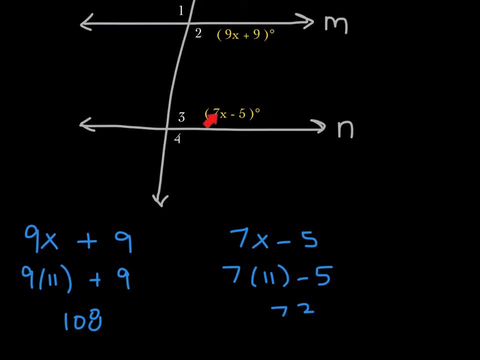 Also the measure of angle 4. And then I found that this expression 7x minus 5 degrees, turns out to be 72 degrees when I plug in 11. So angle 3 is 72 degrees. Alright, cool. 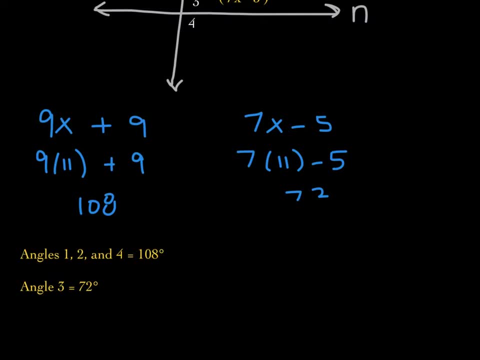 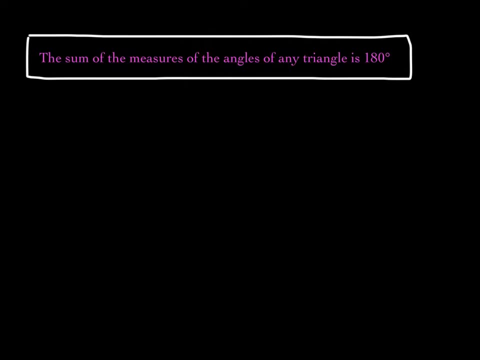 That was pretty fun. Let's go to the next example. Now, going forward in our class, we're going to make use of this important fact many times. The sum of the measures of the angles of any triangle is 180 degrees. Add the three angles of any triangle. 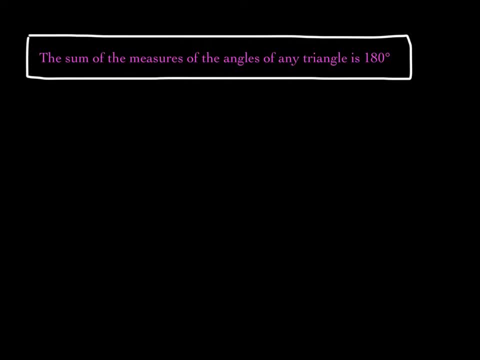 and you will always get 180 degrees. Alright. our next example: Find the measures, or the measures of 2 of the angles of a triangle are 33 degrees and 26 degrees. That word is misspelled there. Alright, find the measure of the third angle. 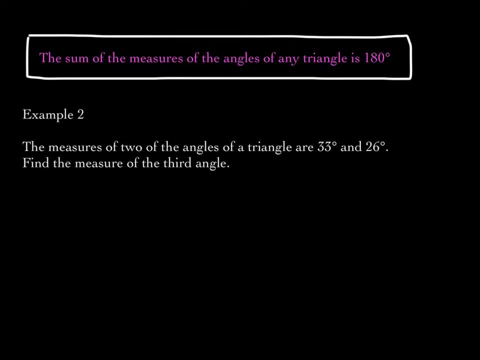 Now we know that the sum of the three angles of any triangle is 180 degrees. So if I take 33 degrees and add it to 26 degrees and add it to my third unknown angle, I should get 180 degrees right. 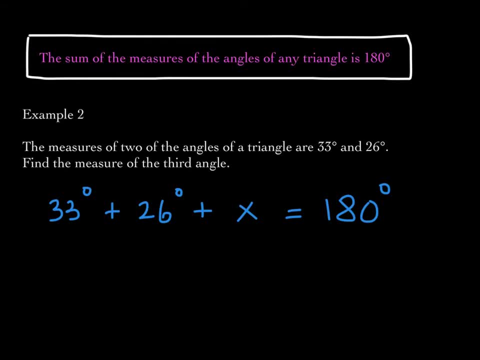 So that's making use of this fact up here Now I can just solve this equation for x. I'm actually going to invite you to pause the video here and solve this equation for x and find the measure of that last, that third angle. 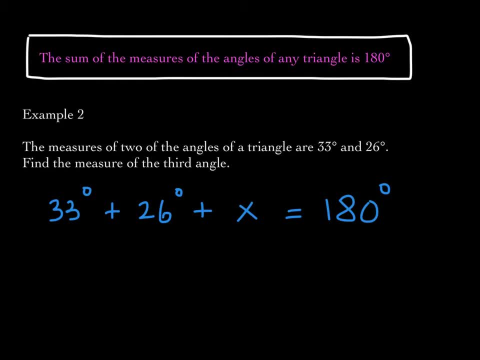 So go ahead and pause the video here, Alright, I hope you paused the video and worked this problem out for yourself, And I hope you and I agree that that last angle must be 121 degrees. Great job, Alright, let's continue studying. 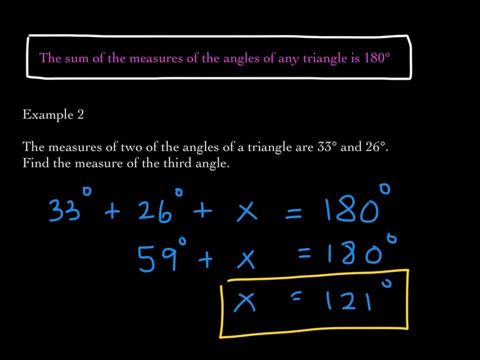 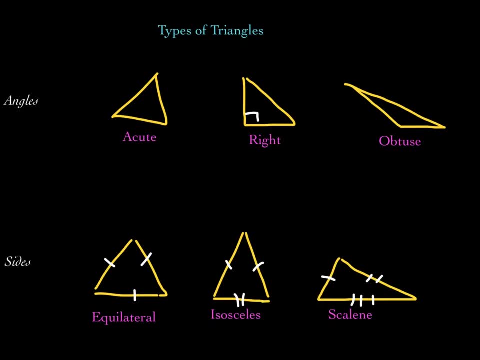 and let's focus our attention now on different types of triangles. Okay, types of triangles. Now we can classify triangles by their angles or by their sides. If all of the angles within a triangle are acute, then the triangle is an acute triangle. 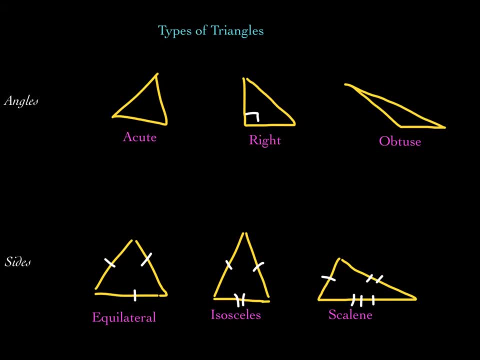 If one angle within the triangle is 90 degrees, then it's a right triangle, And if one of the angles in a triangle is obtuse, then it's called an obtuse triangle. Now, classifying the triangles by their sides, we have an equilateral triangle. 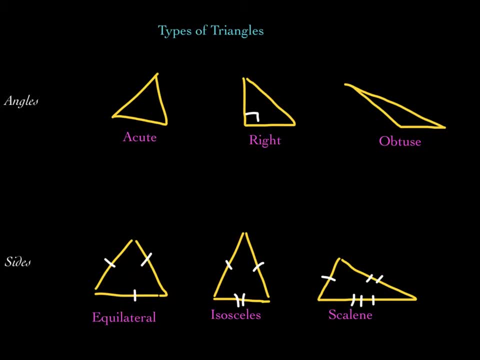 where all of these sides are the same length. An isosceles triangle is a triangle where you have one pair of sides that are equal in length, So these two are the same, these two sides are the same length, And then you have a scaling triangle. 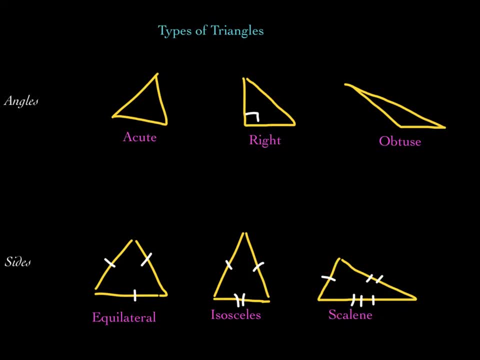 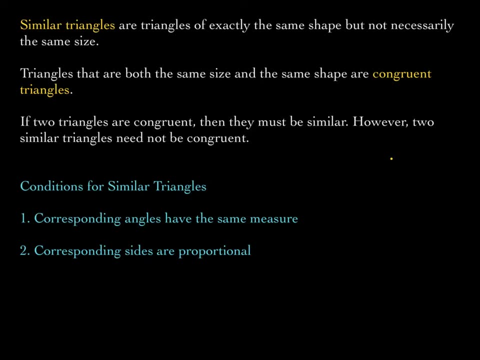 where none of the sides are the same length, So they're all different lengths. Now we have this notion of similar triangles. Now, similar triangles are triangles of exactly the same shape, but not necessarily the same size. Okay, Triangles that are both the same size. 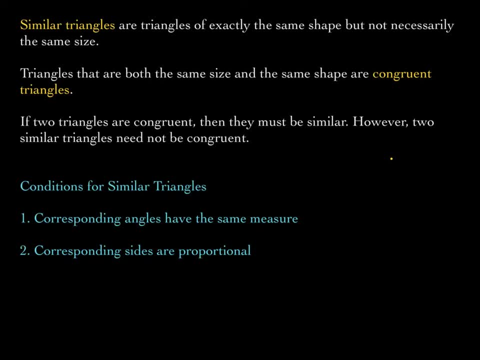 and the same shape are called congruent triangles. So congruency is stronger. It's the same shape and the same size. If two triangles are congruent, then it's possible to pick one of them up and place it on top of the other. 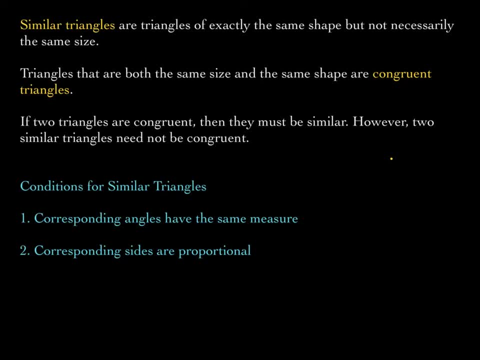 and they will coincide. That's congruency. But similar triangles are not necessarily the same size, but they do have the same shape. Now, if two triangles are congruent, then they must be similar. However, two similar triangles need not be congruent. 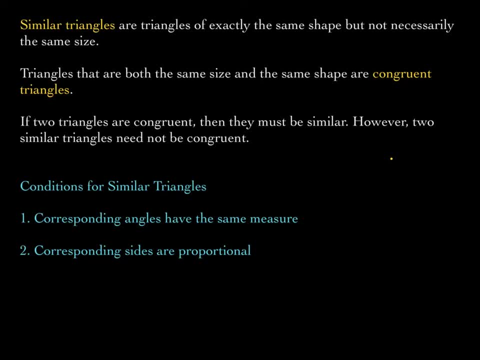 Okay. So if you're congruent, then that means you're similar, But if you're similar, it doesn't necessarily mean you're congruent. Now, two triangles are similar. They can be called similar triangles if the following two conditions are met: 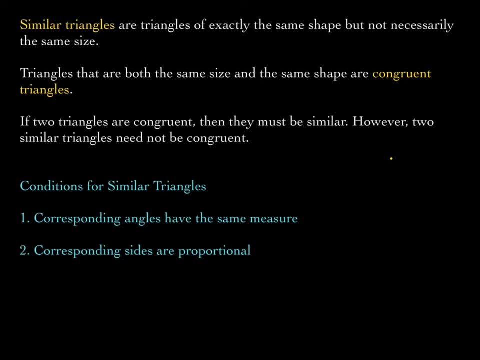 Number one: corresponding angles have the same measure And number two: corresponding sides are proportional. Now, when we say they are proportional, that means the ratios of their corresponding sides are equal, And I'll show you what that means in just a second. 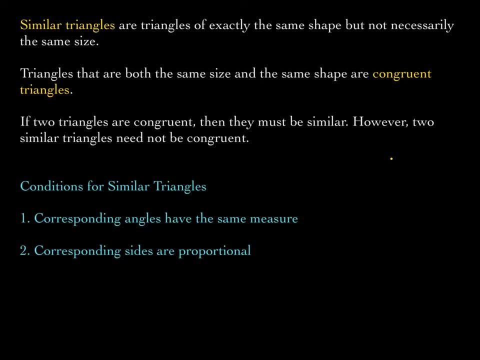 So the only way we can say a triangle is similar to another is if these two conditions are met. Now just remember: similar triangles does not necessarily mean the same size. It does mean the same shape. however. In this example, we have triangles D, E, F and G, H, I. 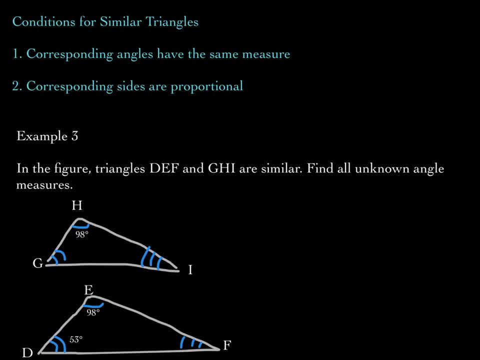 and they are similar. Find all unknown angles and find all unknown angle measures. I think the first angle I would like to find is angle F. I can use the sum formula to find angle F, That is to say 98 degrees plus 53 degrees. 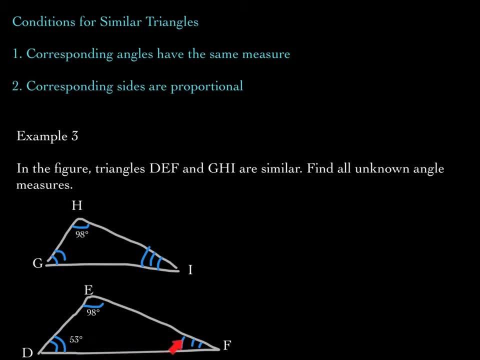 plus angle F must equal 180 degrees. So that leads me to find that F is 29 degrees Now. angle F corresponds to angle I. That means angle I is also 29 degrees Now. angle D corresponds to angle G. 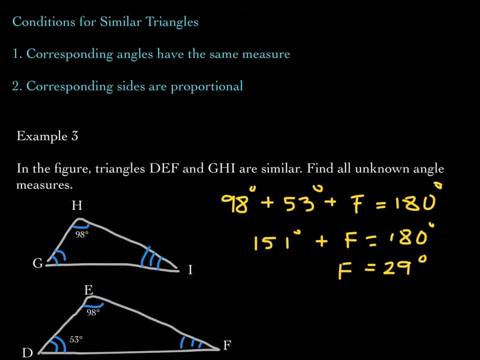 So angle G is also 53 degrees. All right, very good. So then here is our final answer right here, And we used the fact that for similar triangles, corresponding angles have the same measure, So we're taking advantage. 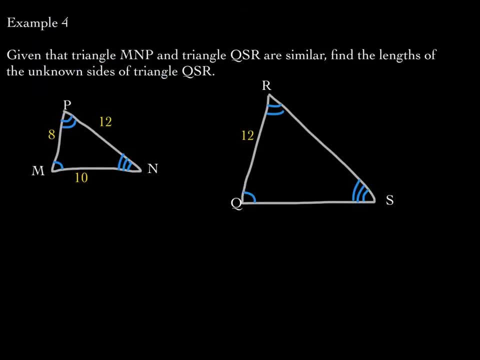 of this first condition here. In this next example it says: given that triangle M and P and triangle QSR are similar, find the lengths of the unknown sides of triangle QSR. All right, we're going to take advantage of the second condition. 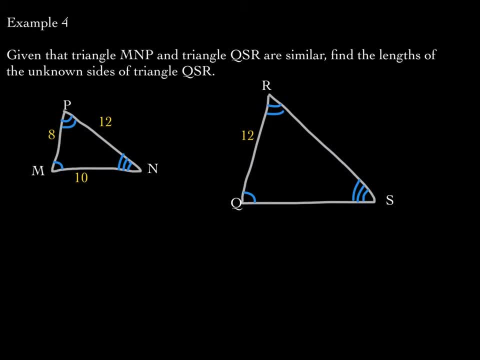 for similar triangles. That is to say, similar triangles have corresponding sides in proportion. okay, So here we go. I am going to. let's see. I need to know what side QS is right. I need to know this length. 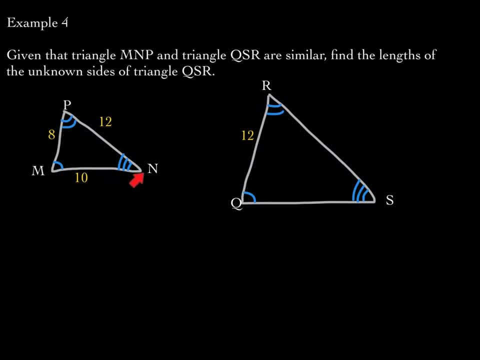 Now, side MN corresponds to side QS. Side MN corresponds to side QS. Furthermore, let's see: side MP corresponds to side QR, right? So I can say the following: MN is to QS, what MP is to QR? I'll say that again. 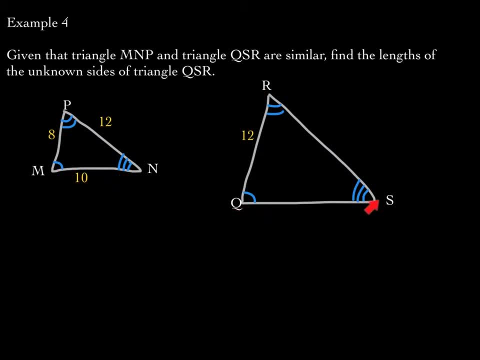 MN is to QS, what MP is to QR, So I can set up a proportion that looks like this. So this, you guys, is called a proportion. A proportion is a statement that two ratios are equal. So here is a ratio. 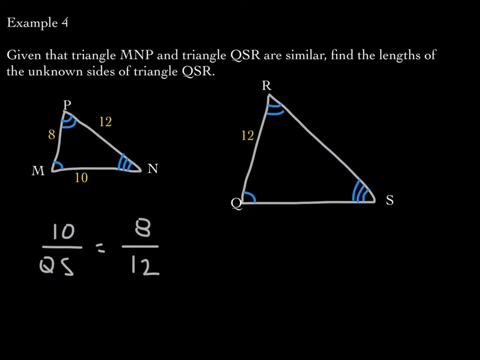 10 over this side must be equal to 8 over this side, And then I can cross, multiply to find the unknown. So I can do this right Now. it might be easier. actually, I'm going to go back for a second. 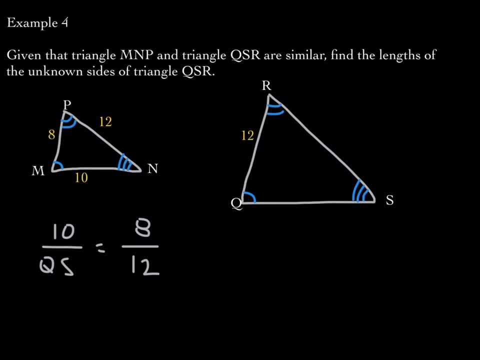 It might be easier- I'm not sure- if we simplify this fraction first. So the GCF between 8 and 12 is 4.. So I'll divide both 8 and 12 by 4 to give me 2 thirds. 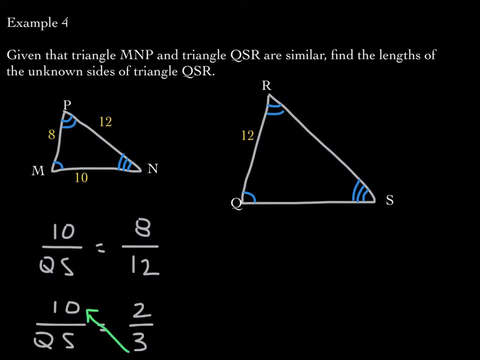 So now I will cross multiply. You didn't have to simplify, but it did. it's going to make this a little easier for us. So now we have: 2 times QS must be equal to 10 times 3, which is 30.. 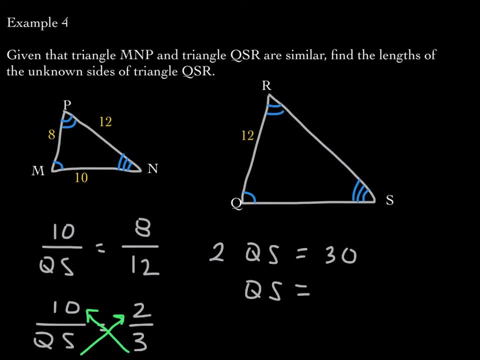 Dividing both sides by 2 gives us that side QS is equal to 15.. Alright, so I know this side length here I got it. it's 15.. Now, the only side length that's missing is RS, RS. 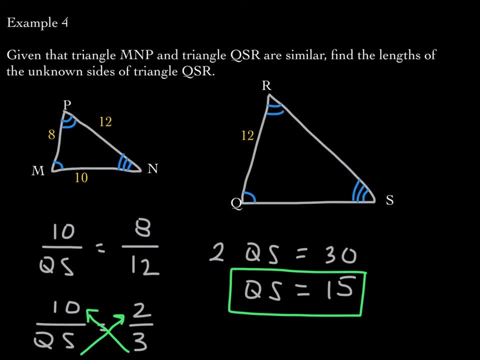 So I'm going to set up a brand new proportion, okay, Actually, I'm going to invite you to pause the video and set up a brand new proportion and solve for RS. please Set up a brand new proportion and solve for RS. 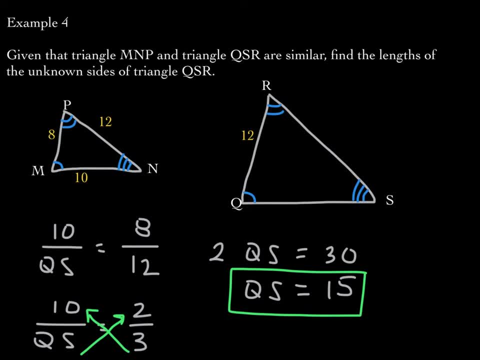 So go ahead and pause the video here, would you, And finish that off for us. Alright, everybody, I hope our results match. I set up a brand new proportion. I did 12 is to 8, what this unknown side is to 12.. 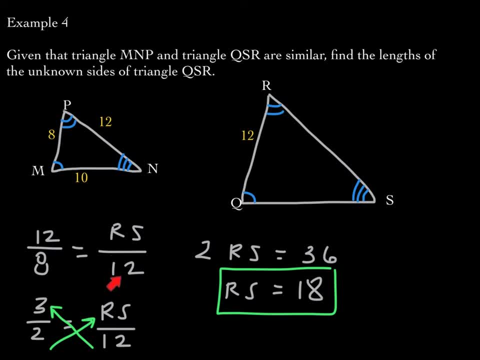 12 is to 8, what RS is to 12.. I also simplified 12 over 8 to be 3 halves. before I cross-multiplied, That's optional. At the end of the day, you should find that RS is equal to 18.. 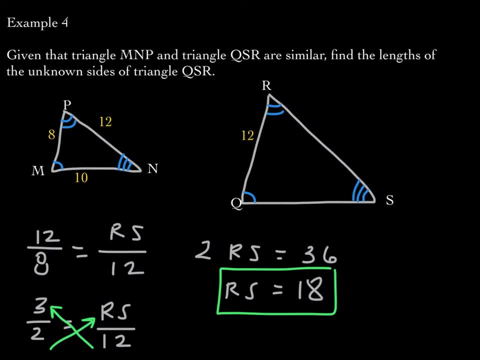 I want to call something out here before we move on: Do not simplify across the equal sign. So do not think that these 12s cancel out. That would be incorrect, okay. So please do not do that. Also, right here: this 3 and this 12,. 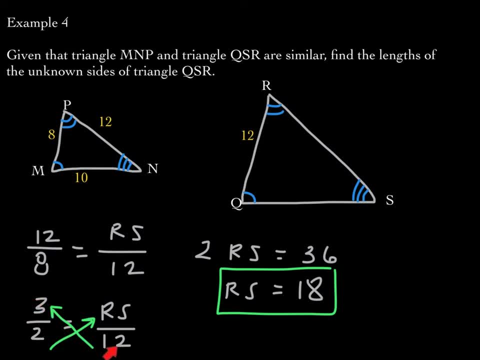 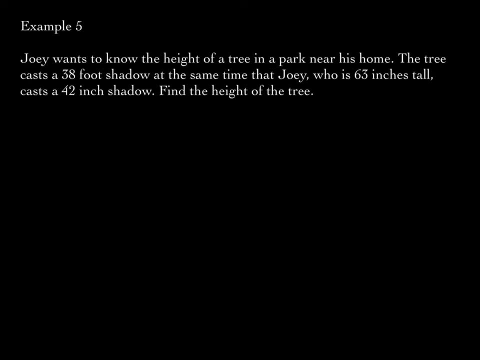 do not divide 3 into 12, like you're cross-canceling. You cannot do that across an equal sign, so be very careful. Alright, cool, Alright. our last example here: Joey wants to know the height of a tree in a park near his home. 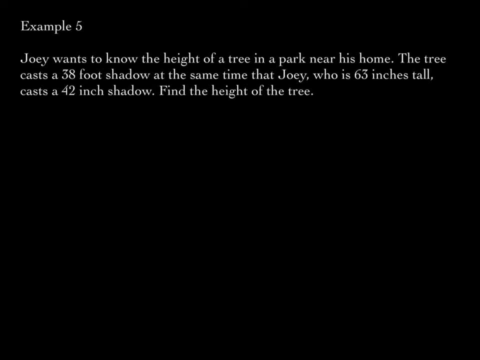 The tree casts a 38-foot shadow at the same time that Joey, who is 63 inches tall, casts a 42-inch shadow. Find the height of the tree. I think what is best here is for us to draw a picture, so let's do that. 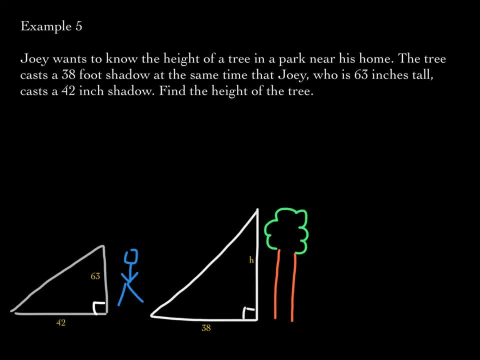 Alright, here's my fancy drawing. everybody, Aren't I the artist? right? If you actually look back at my kindergarten or first grade like diagrams, I have not progressed at all. I still do stick figures and my trees look the same. 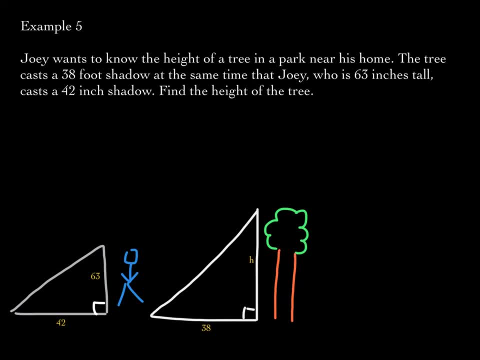 So, anyway, it's not really about the fancy drawing, It's about getting an accurate picture of what's really happening in this story. So here's Joey, Hi, Joey, And Joey is 42 inches. I'm sorry, no, he's not. 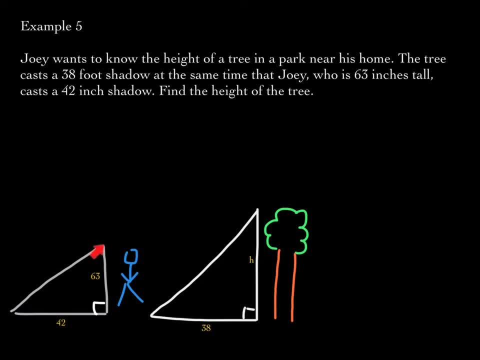 He is 63 inches tall and he casts a 42-inch shadow. The tree here casts a 38-foot shadow and we don't know the height of the tree, and that's what we're trying to find. So why don't you go ahead and pause the video here?